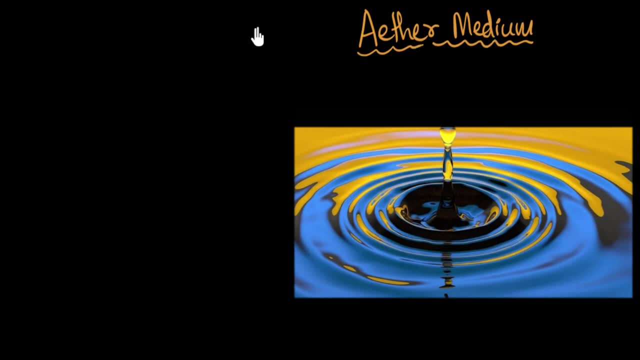 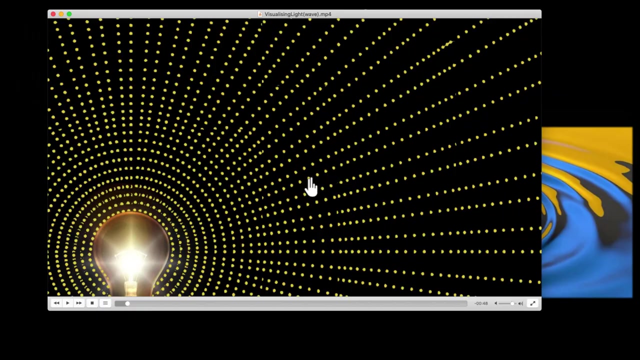 Light is. you know, light waves are carried by the vibrations of the aether medium, So light is propagated by the vibrations of the aether medium. Now, if you want to visualize something like that here, here's our animation, Here's our light bulb and these particles. 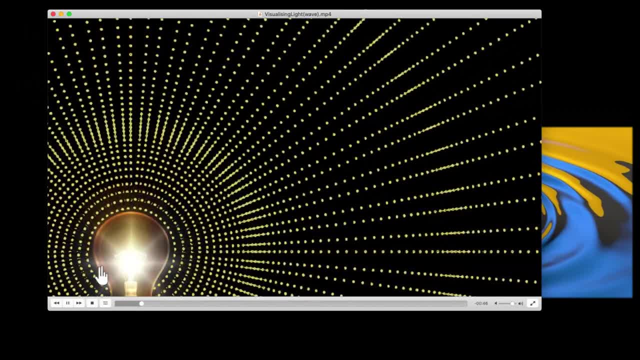 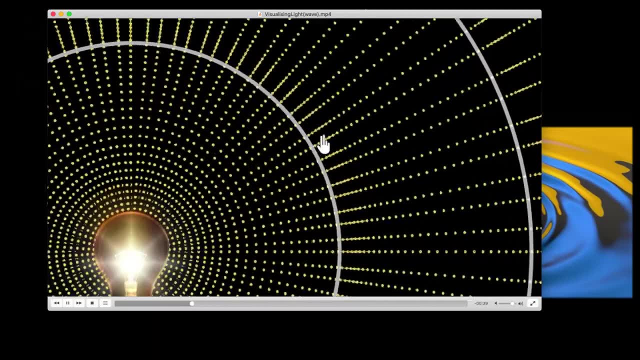 are the particles of the aether medium that's present everywhere in the universe, And this is how Huygens imagined it. Light is basically disturbance propagated by the vibrations of the aether particle Ripples. Light is ripples in the aether medium. 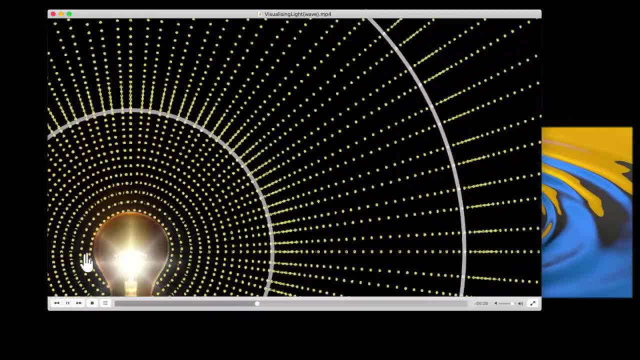 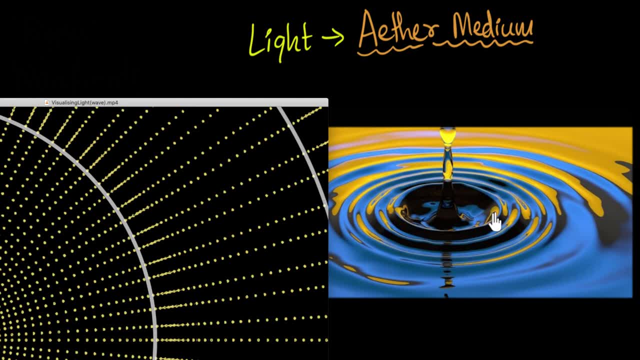 Beautiful, right. Well, now there's one difference, big difference, between the ripples of light and the ripples of water, Water, Water, Water. These ripples are on the surface, which is 2D, 2D, two dimensions. 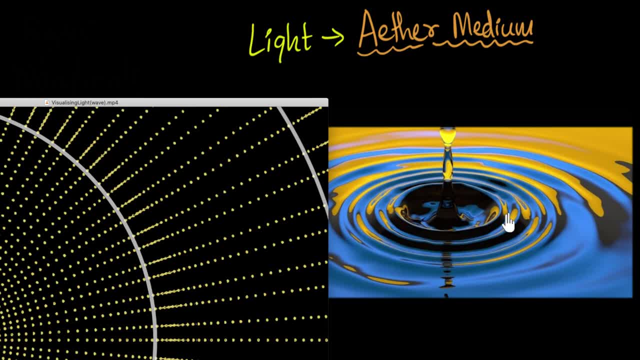 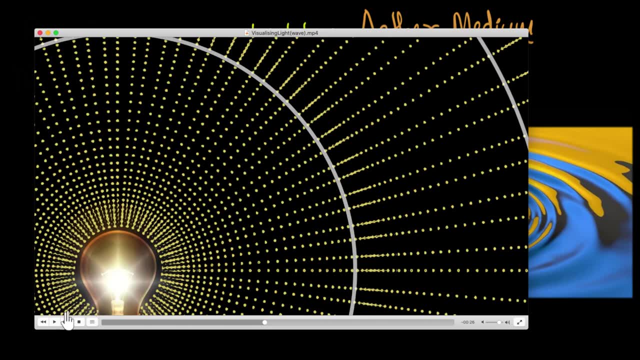 And so these ripples are indeed circular, and you may have seen them, But light is a wave in three dimensions, So, although you can't see this in this diagram, it's in three dimensions. so these ripples are not circles, but these are spherical ripples. 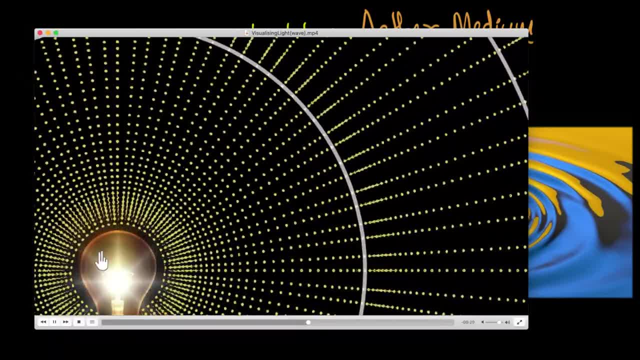 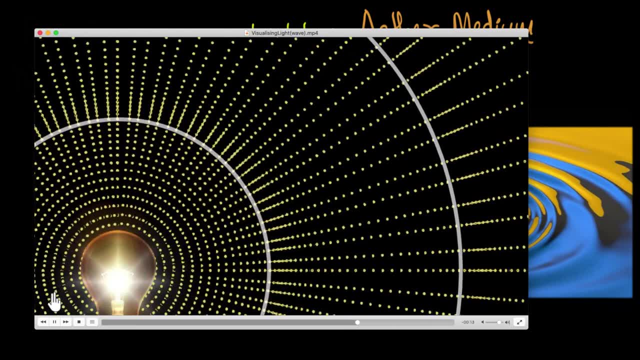 That's a major difference that you're finding. So this is a 3D wave, But now we can ask a question. We can ask: what exactly are these ripples? Whether you consider light or whether you consider water, what exactly are those ripples? 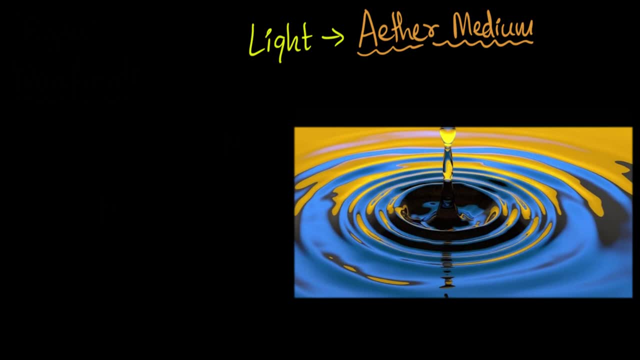 So let me get rid of this and talk about that. So what exactly are these ripples? Well, in physics, these ripples have a very technical and fancy name: We call them wavefronts, And you'll keep hearing this word over and over again. 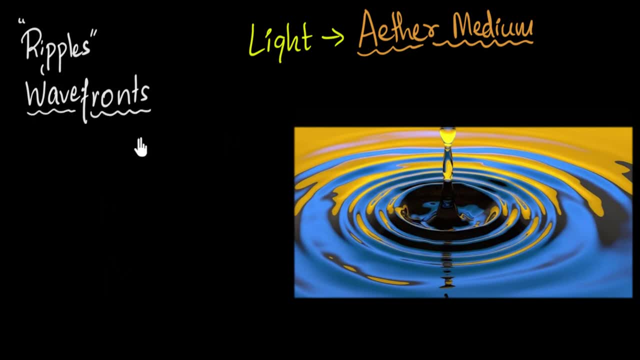 in the future videos. So let's clarify what these wavefronts are. Well, wavefronts, let me just define them first and I'll show you. Wavefronts are basically set of particles. Wavefronts are basically set of particles. 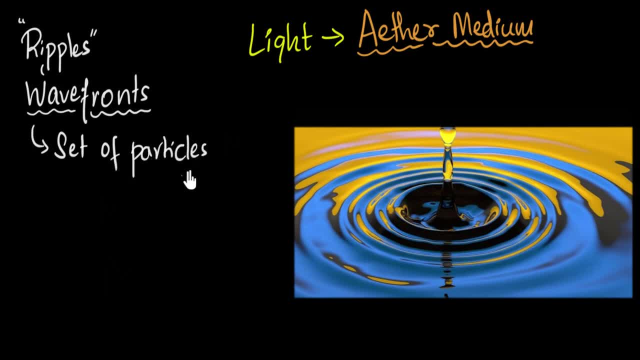 Wavefronts are basically set of particles which are in sync with each other, which are vibrating in sync, And again, there is a technical term for particles vibrating in sync with each other. We call them in phase with each other. We just need to familiarize ourselves. 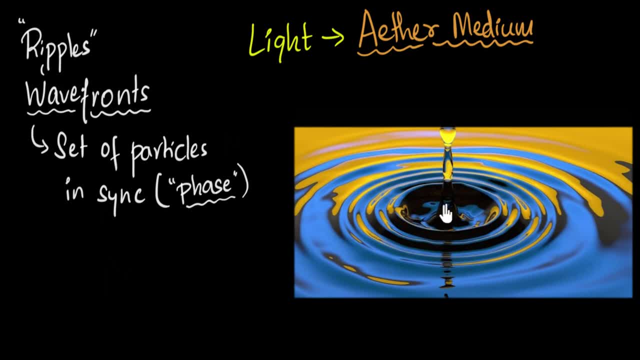 with these technical terms. So what do I mean by this? Well, if I come over here and look at one of these ripples or wavefronts and concentrate just on them, what I will find now is that. what I will find now is that. 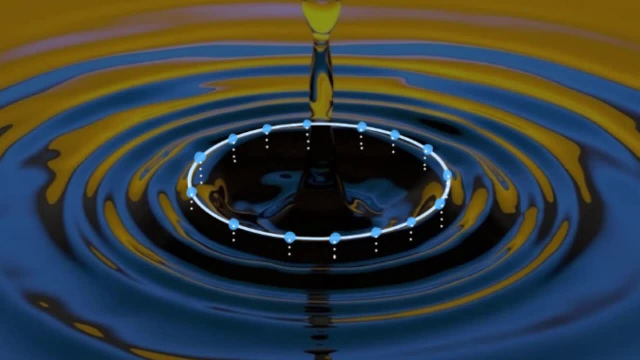 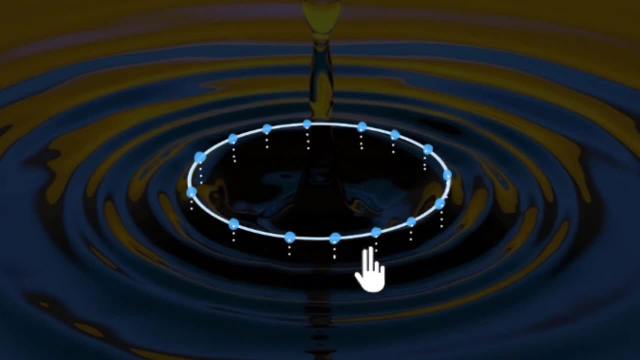 every particle on that ripple or on that wavefront is at the topmost position And that's why that ripple is a crest. A little later in time we'll find all those particles will be at the bottom most position, forming a trough. Let me show you one more. 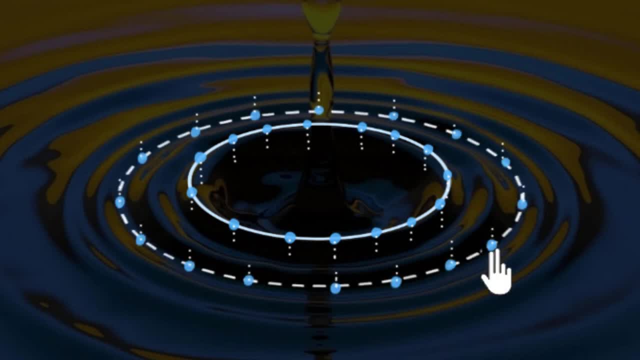 which is already a trough. over here We usually denote trough by dotted lines: A trough. if I look at that particular ripple then you'll find all the particles on that are at their bottom most position. are at their bottom most position. The important thing to note is that 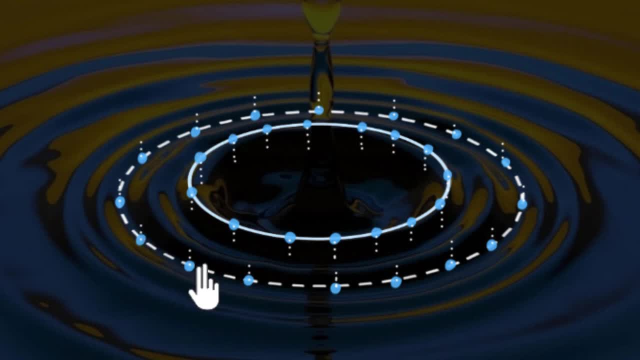 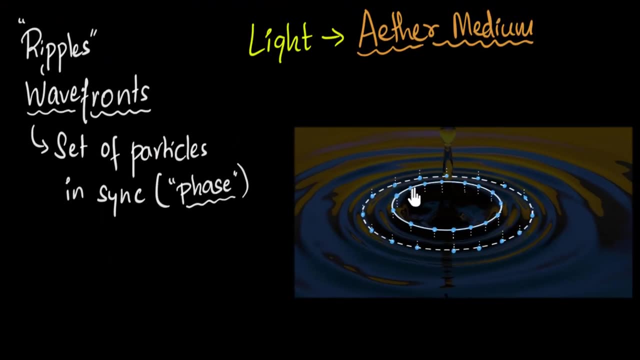 all the particles on these circles. they are always vibrating in sync with each other. They're vibrating together, in phase with each other. Such a set of particles is what we call a wavefront, And the same would be true for our light as well. 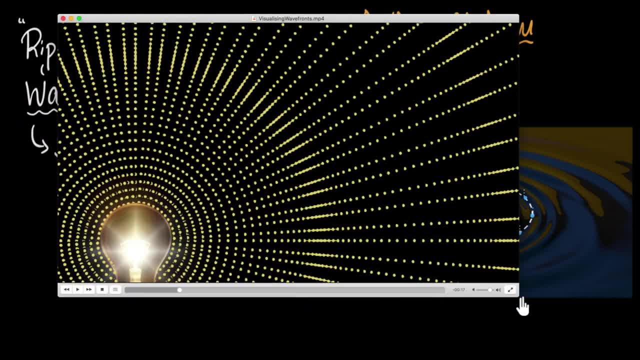 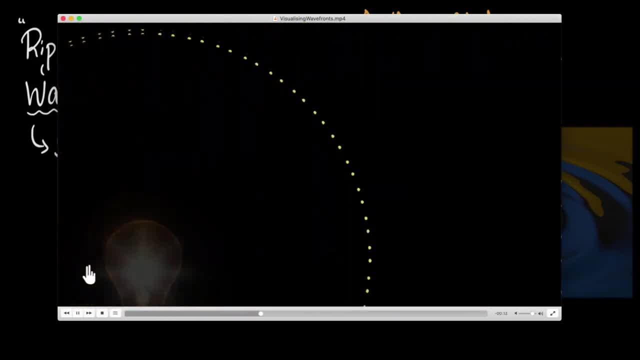 Again, let me bring back that visualization. If I were to concentrate on one of those spheres and just look at those spheres, what you are finding now is: look, all the particles on that spheres are vibrating in sync with each other. You see that. 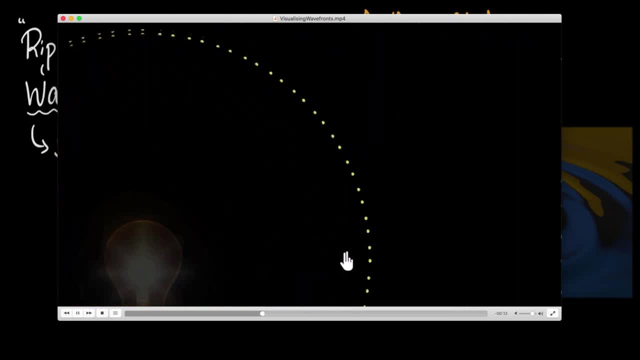 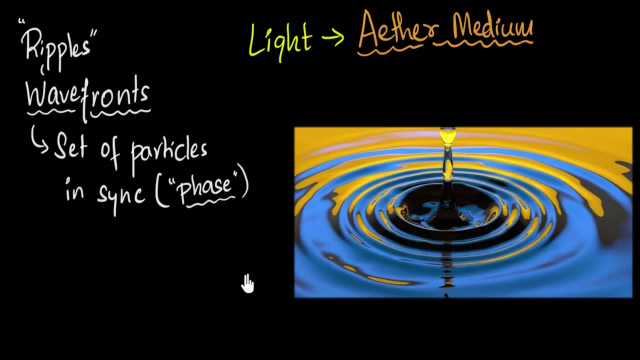 Look at it one more time. All right, there you go. Look at that. They're vibrating in sync with each other. Such a set of particles which are vibrating in sync with each other are what we call wavefronts. The last question I want to explore is: 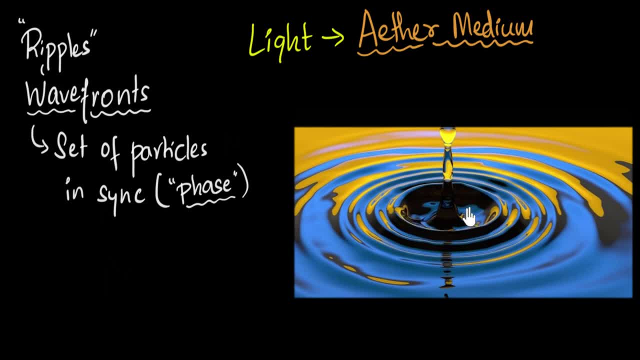 what, in general, would be the shape of these wavefronts? Well, think about water first. If you were to disturb it at only one place, at just one tiny spot, then you'll get these nice circular ripples, or circular wavefronts. 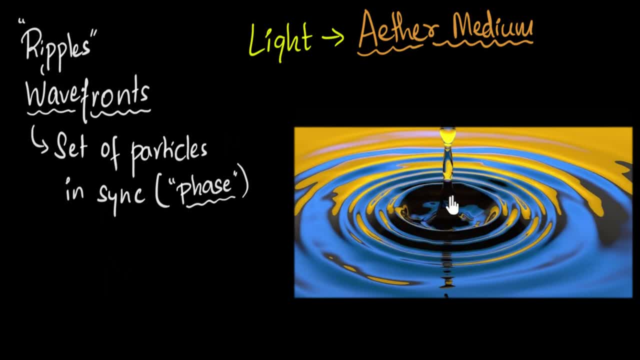 But if you were to disturb this all around with your hand everywhere, then the wavefronts are gonna be all messed up and we'll have weird shapes right. Same would be the case with light as well. Again, looking at that animation, 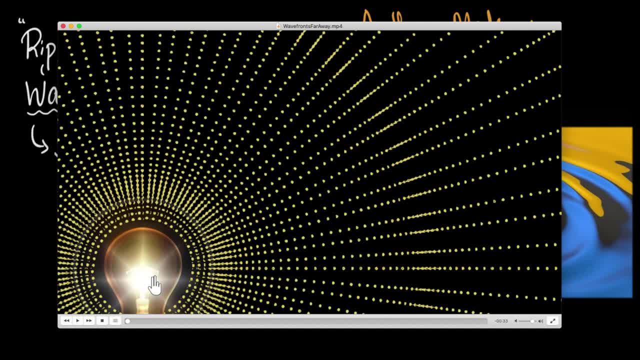 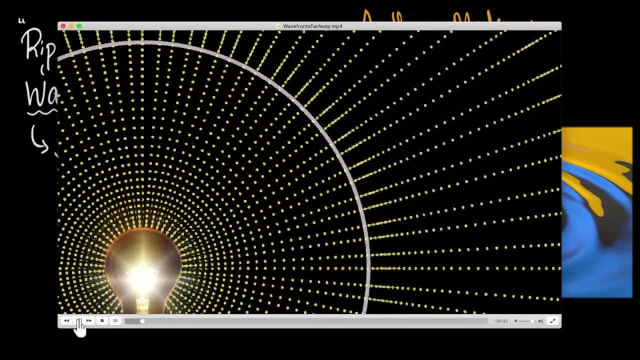 If the light source that we're dealing with is pretty tiny, or we're looking a little bit far away so that the bulb appears tiny, then the wavefronts are going to be spherical in nature, just like those ripples. But if you were to have a big source, 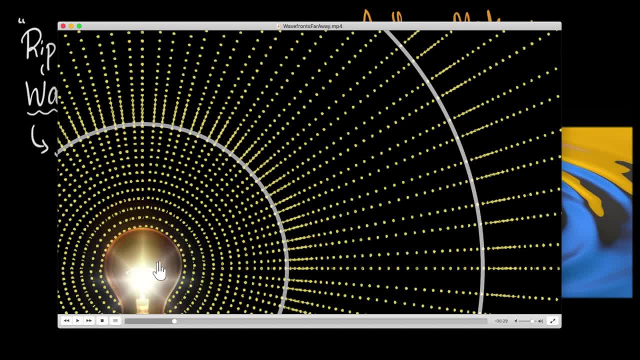 or if you were to go very close to that light bulb where you can no longer neglect the size, the very close to that light bulb. the wavefronts won't be spherical. They might have different shapes depending upon the shape or the size of this light source. 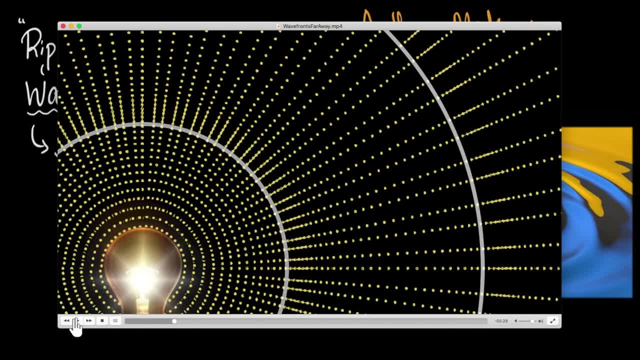 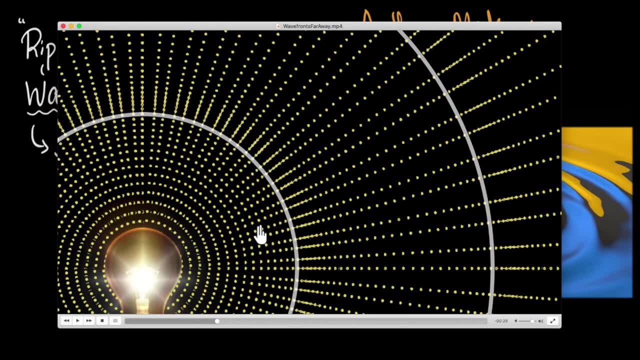 But if you go far away, a little bit far away, where it appears to be a point, then the shape is gonna become spherical. But I want you now to pause this video and think a little bit about what would be the shape of the wavefront. 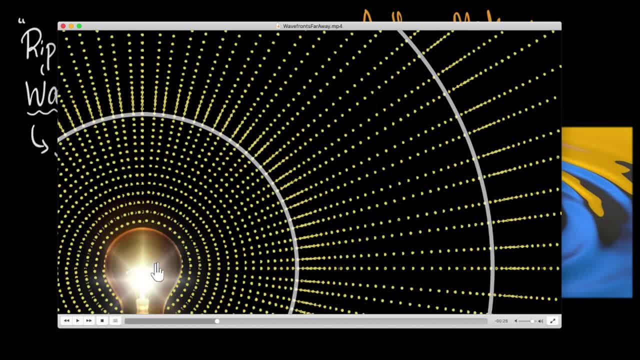 if you were to go really really far away from this light bulb? Think about that. That sphere is gonna become really really big. What now would be the shape of that wavefront? Can you pause the video and think a little bit about that? 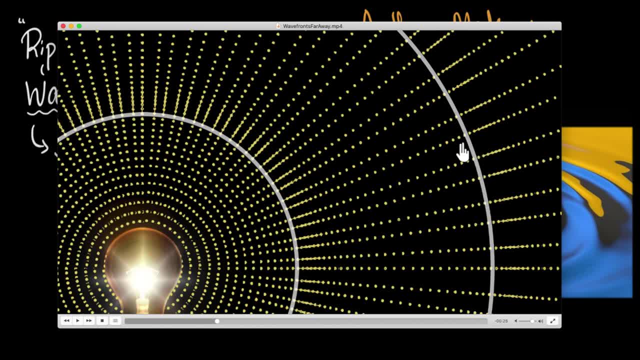 All right, If you were to go really far away, that sphere would become so big that the sphere would appear flat to us, just like how Earth appears flat to us when we look at it from a small distance. right, So let me show you that. 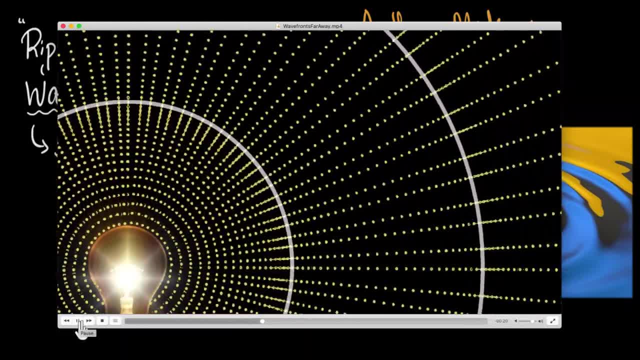 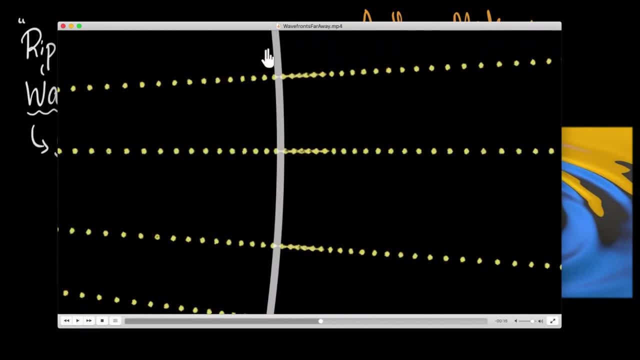 If you were to go really far away from this- and we'll do that in a second. Now, there we go. If we go really far away, I go really really far away- then look at this. This is a sphere of course. 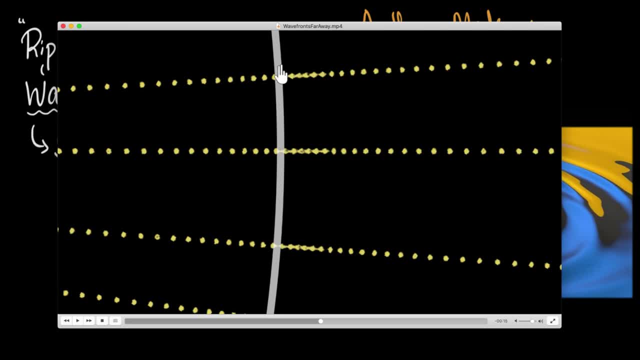 but what we are seeing now is not a line, It's- remember, it's in three dimension, It's flat surfaces. So now we are getting flat ripples, Or flat or plain wavefronts, That's what we call them. 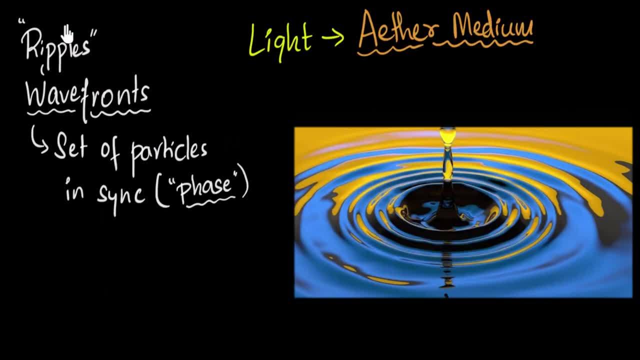 Plain wavefronts. okay, So usually, what would be the shape of these wavefronts? Well, if you're dealing with, say, point sources, point sources, then the shape is going to be spherical, as we saw. 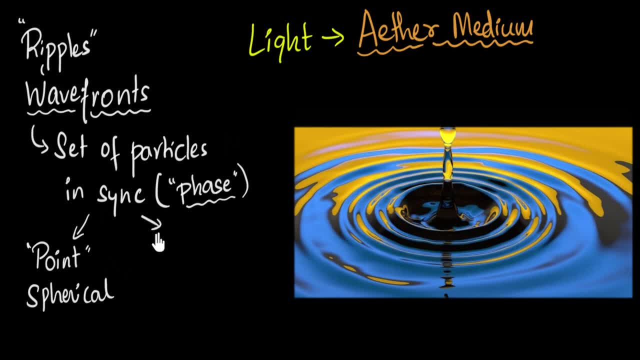 In 2D they are going to be circular, But if you're dealing with point sources or sources which are very far away, you can think of them as infinitely far away. So sources far away, sources far away, then the wavefronts. 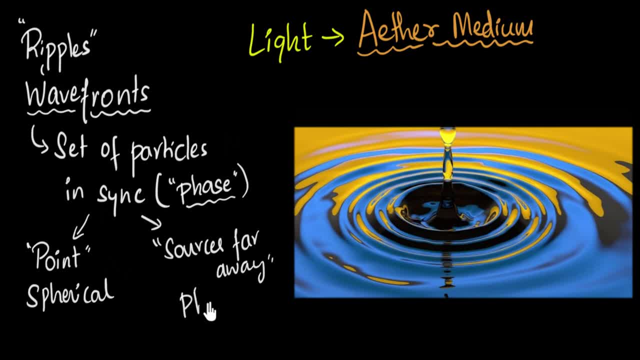 the shape are going to be. the shape is going to be plain. They're going to be flat, flat wavefronts. So the light that we're getting from the sun, for example, on the Earth the light is so far away from the sun.